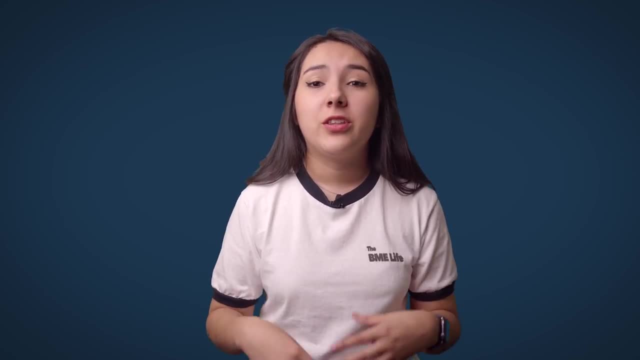 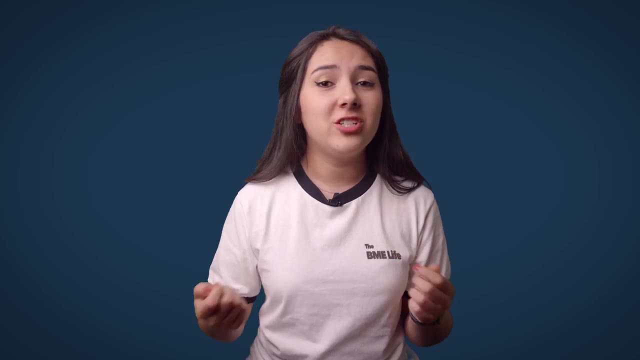 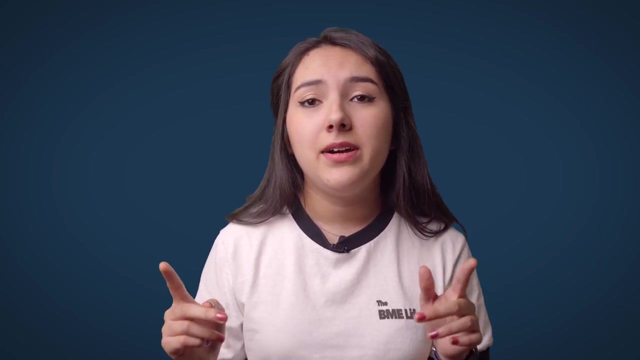 and bioengineering. The short answer is that, although there are indeed technical differences between both, bioengineering and biomedical engineering are used interchangeably and overlap in so many areas. So I'm going to try to elaborate on their differences, but be aware that there's a 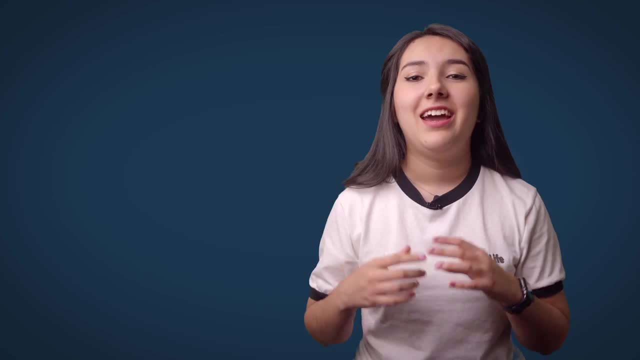 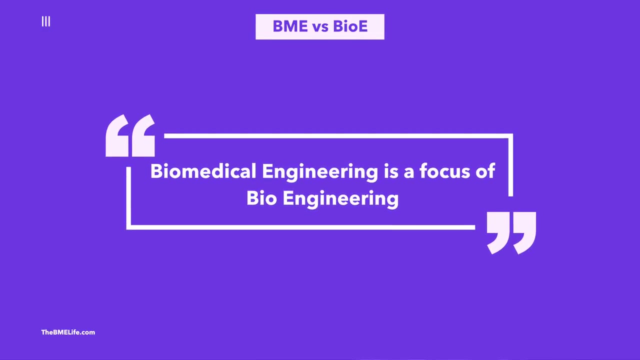 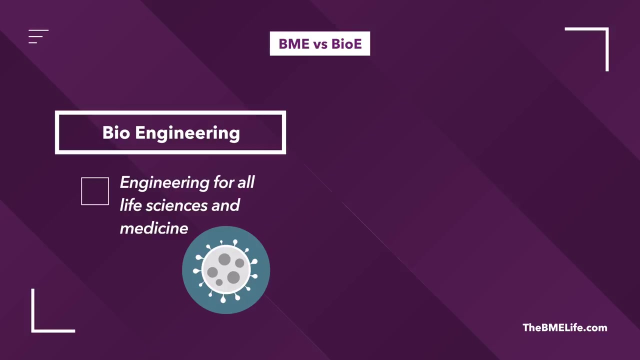 lot of overlapping, which can make it a little bit confusing. An easy way to think about these two majors is that biomedical engineering really is a focus of bioengineering. Bioengineering uses engineering principles to solve problems in all life sciences and medicine, while biomedical engineering focuses on medicine and health care. 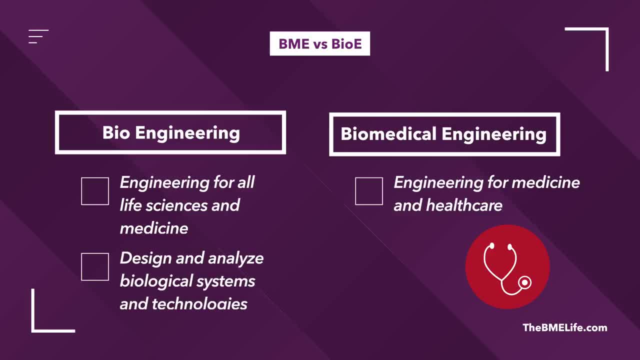 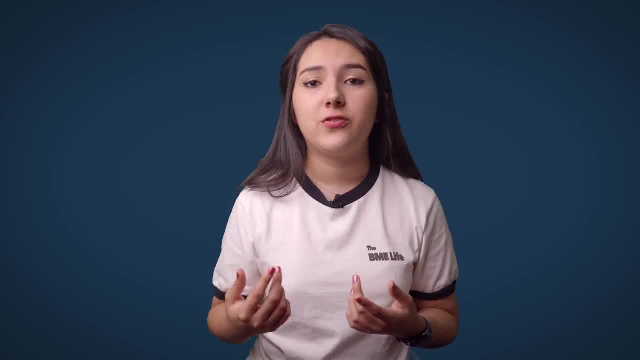 Bioengineering is an engineering discipline that uses its principles to design and analyze biological systems and technologies. Some examples of research focus include engineering bacteria to produce chemicals, tissue engineered organs and pharmaceuticals. Think of bioengineering as a broader field, as it also covers topics outside of medicine, such as. 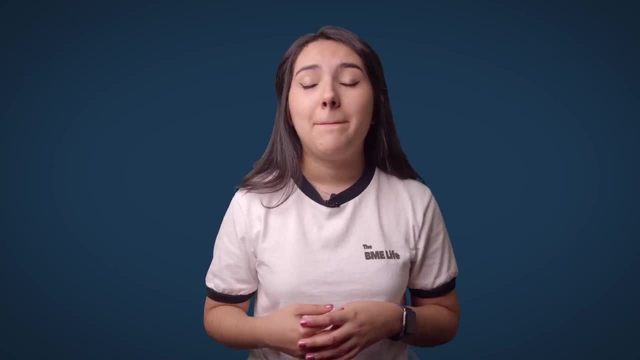 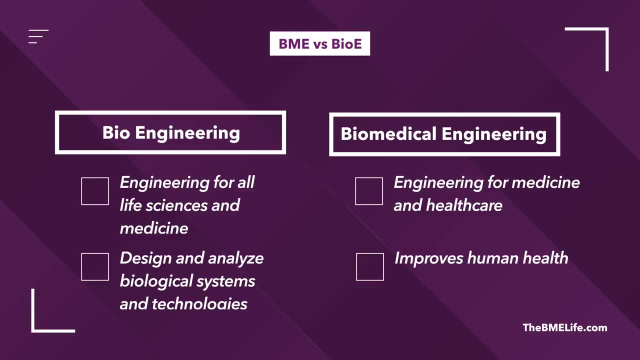 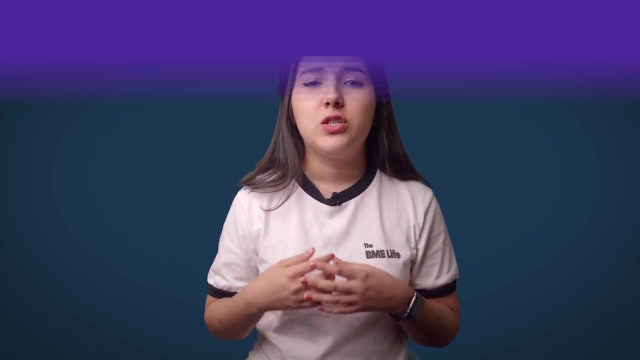 agriculture, natural resources and the food industry. Biomedical engineering is a more complex field which highly focuses on using engineering principles to improve human health. Some examples of BME fields include medical devices, biotechnology and biomechanics. So when you think of 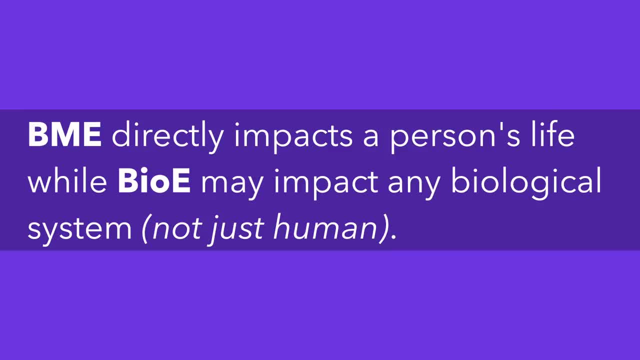 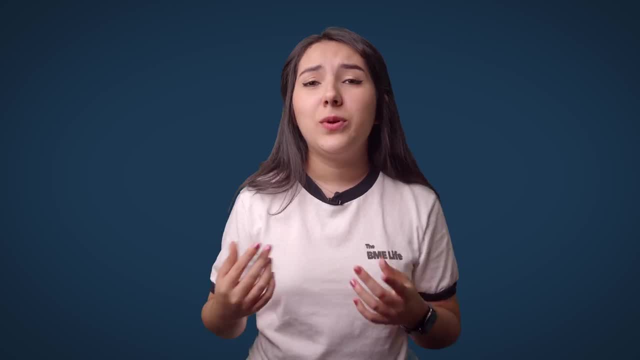 BME, think of technologies and research that will directly impact a person's life, whereas bioengineering may impact any biological system outside of the human kind. So when it comes down to choosing between the two, it is really up to you and your interest to decide. 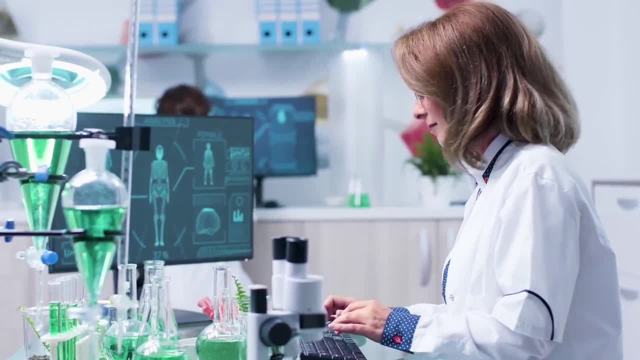 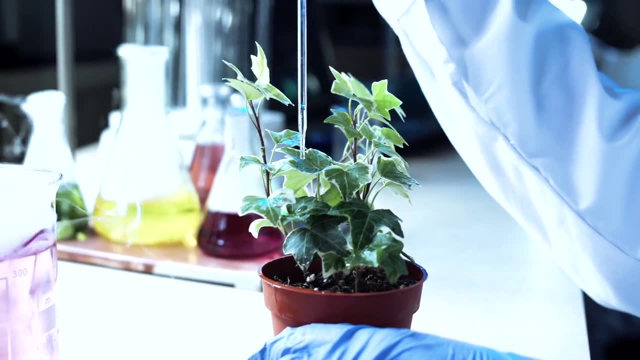 If you would like to learn more about the broader picture and see how you can use engineering to solve problems in medicine and biology, then bioengineering may be a better fit for you. However, if you are interested in improving the healthcare field through medical innovation, 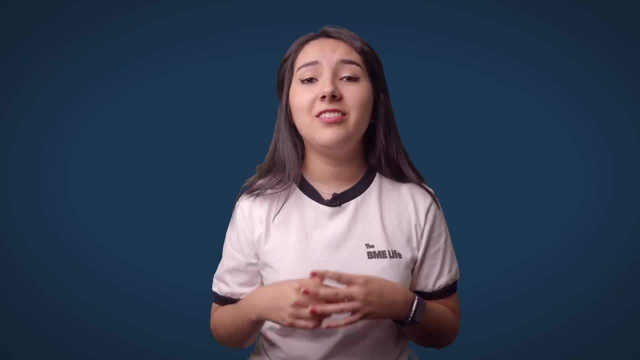 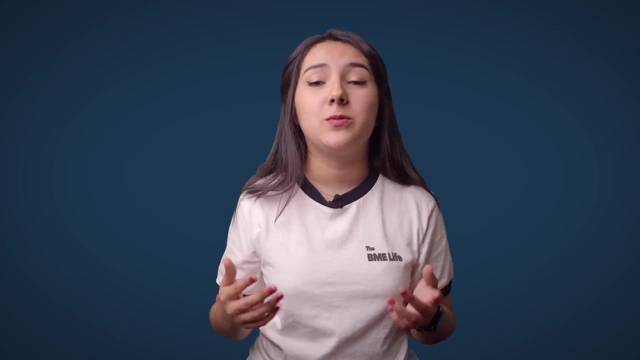 then biomedical engineering might be a better option for you. The reality is that, although there are technical differences, when it comes down to it you can end up doing the same kind of jobs with both of them. Just as you go into the medical device industry as a bioengineer, you can also go into the food. 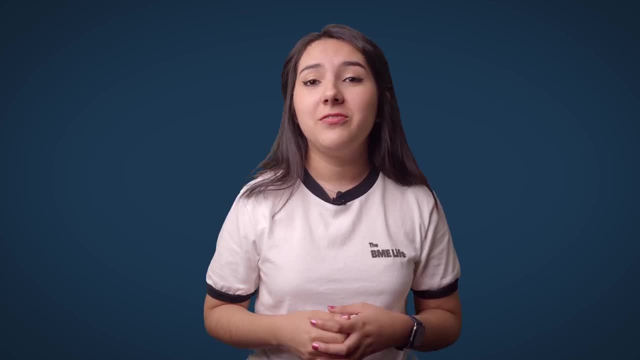 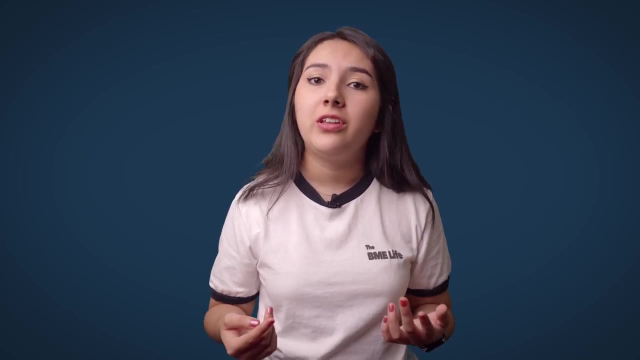 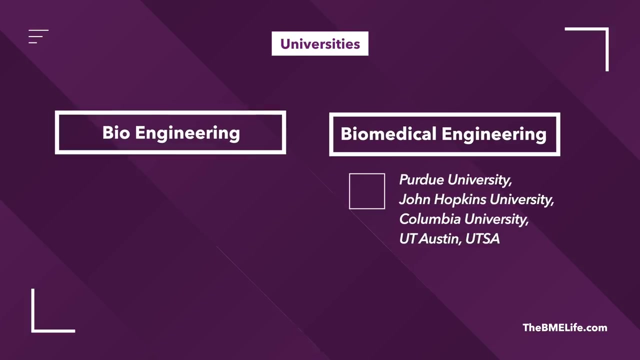 industry as a biomedical engineer. In fact, most universities don't really strictly adhere to their separate definitions and often only offer one degree or the other. Some universities that offer biomedical engineering programs are Purdue University, Johns Hopkins, Columbia University, UT Austin and, of course, my alma mater, UTSA. Similarly, some universities that offer 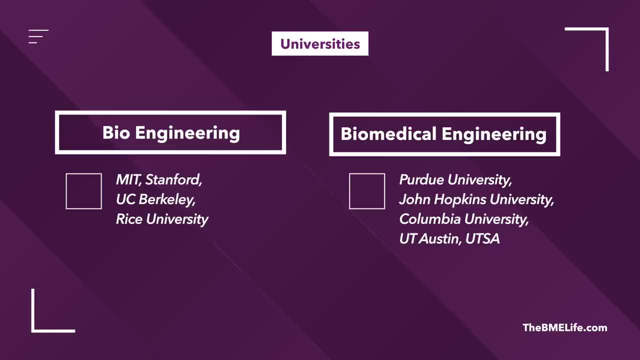 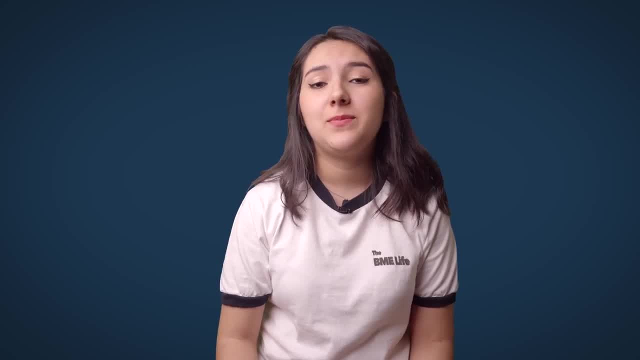 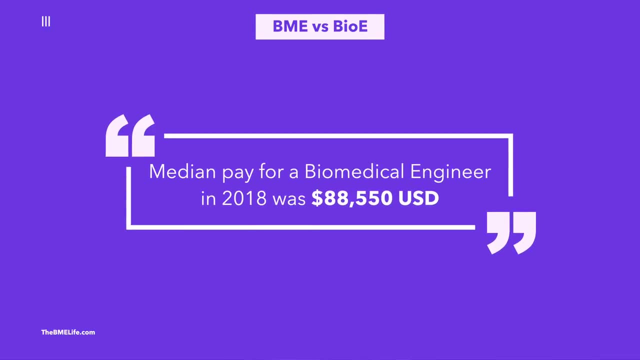 bioengineering programs are MIT, Stanford, EZ, Berkeley and Rice. When it comes to the job outlook, the Bureau of Labor Statistics actually only tracks biomedical engineers, whose median pay in 2018 was $88,550 per year. However, according to ZipRecruiter, biomedical engineers actually 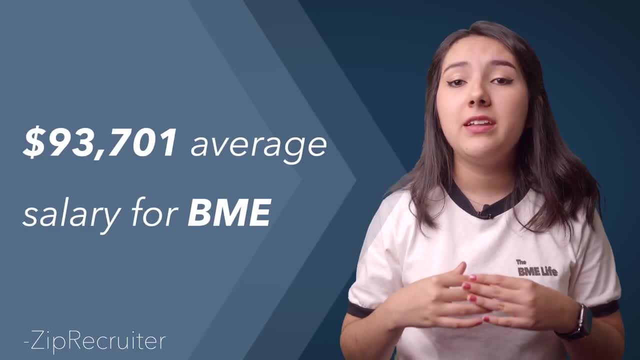 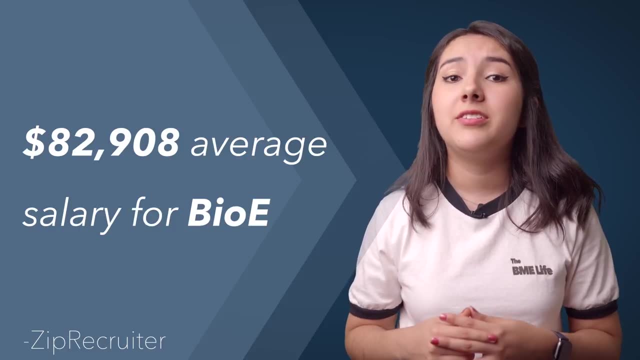 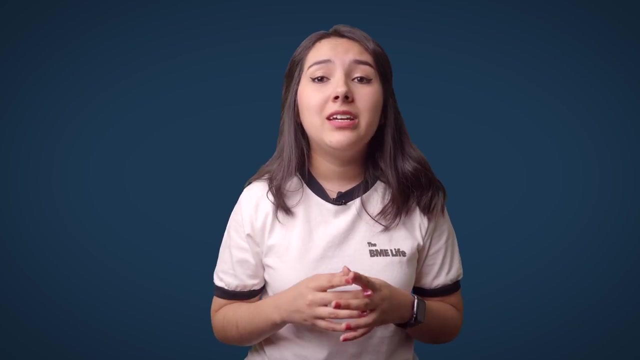 make a little more money than bioengineers, With an expected average of $93,701 compared to a bioengineer's average of $82,908.. This is not to say that bioengineering is inferior in any way, because, again, they really both overlap and you. can get the same kind of jobs with both. Both degrees are a part of a growing industry, but technology in the medical field is definitely growing faster. So before wrapping up this video, I want to say that I personally wouldn't break my head around the differences between these. 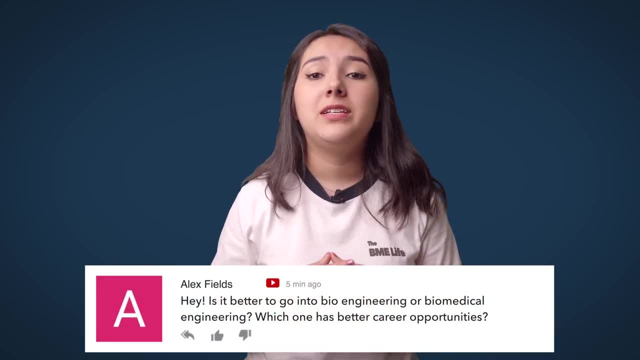 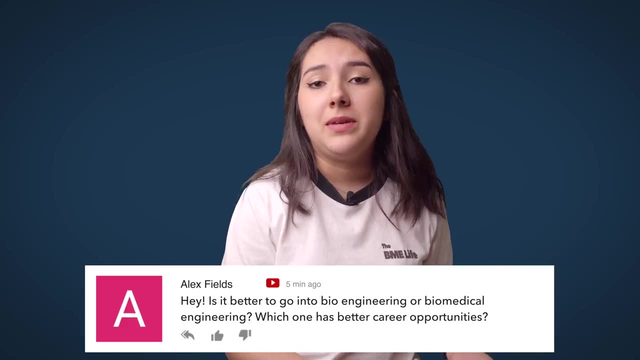 two degrees. If you're interested in learning more about bioengineering, you should definitely take a look at this video, And I say this because I know we have gotten messages about people saying that they're in a school that offers bioengineering but they're not sure if they should be doing BME. 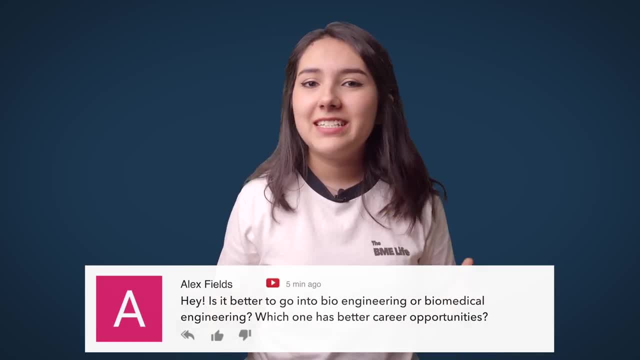 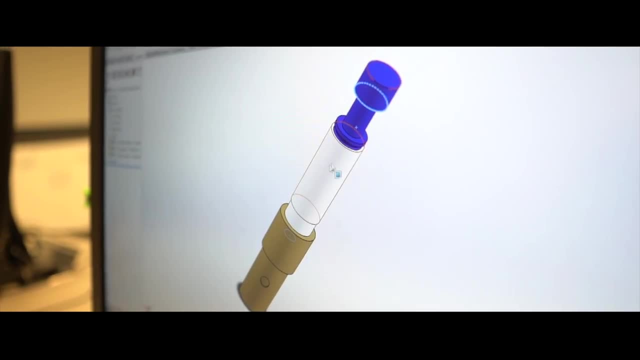 instead, or vice versa. The truth is that it really doesn't matter. And just to give a real world example, in the beginning of this year I actually participated in a medical device make-a-thon where lots of different universities came to participate in a competition where we 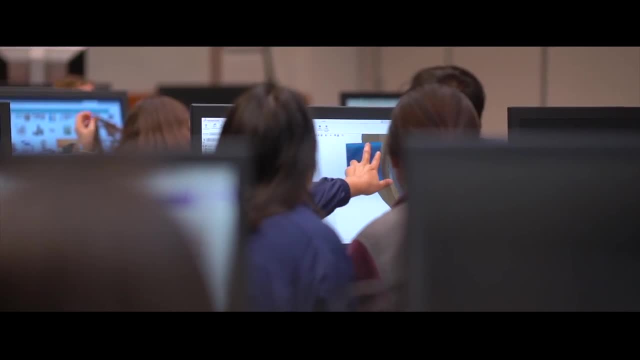 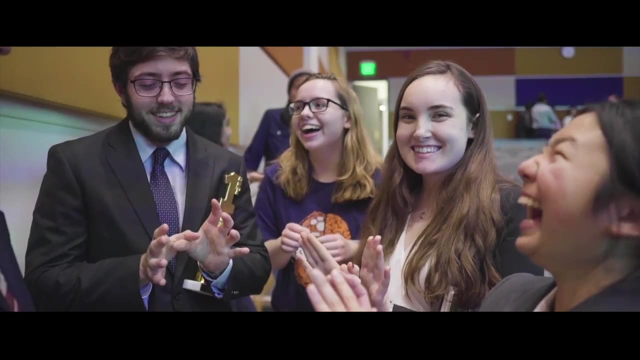 had to come up with a medical device solution to a medical need. One of the participating schools that came was Rice University, and at Rice they offered the bioengineering program rather than BME. The Rice students killed it and knew so much about the medical device industry. 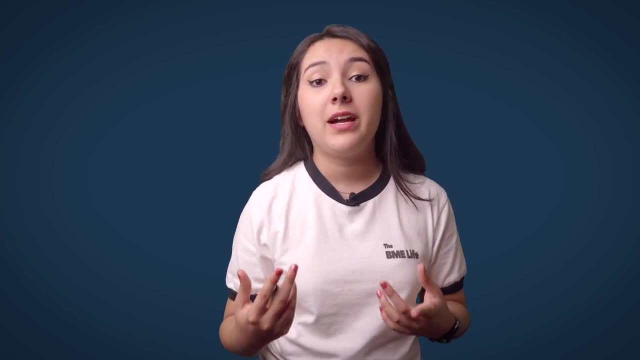 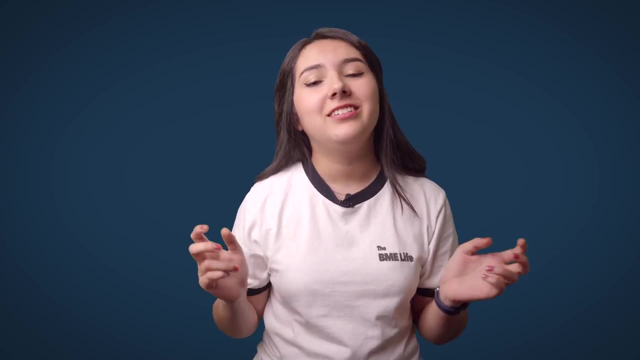 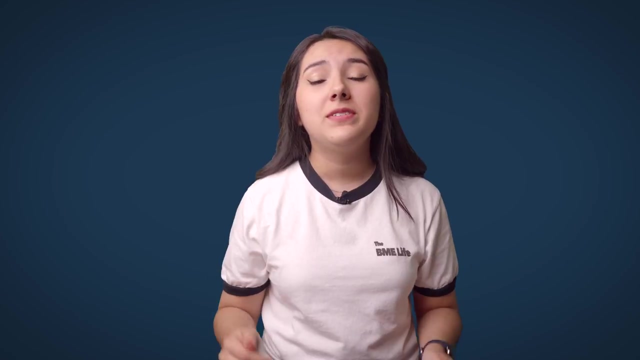 and FDA regulations. So they are a great example that bioengineers can also focus in the medical field if they choose to do so. So, in summary, yes, they are technically different. Bioengineering is a broader field that covers all biological systems, while BME focuses in medicine and